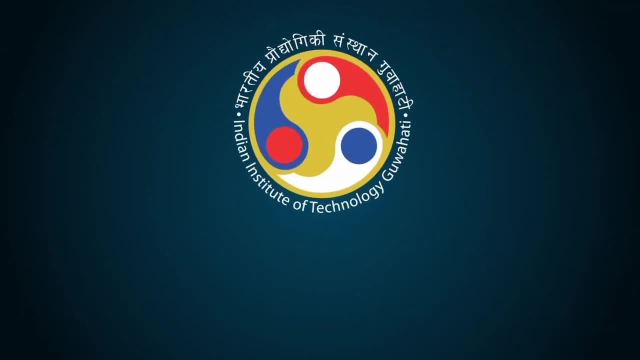 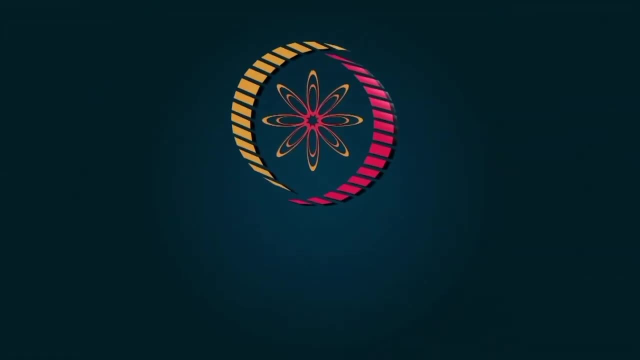 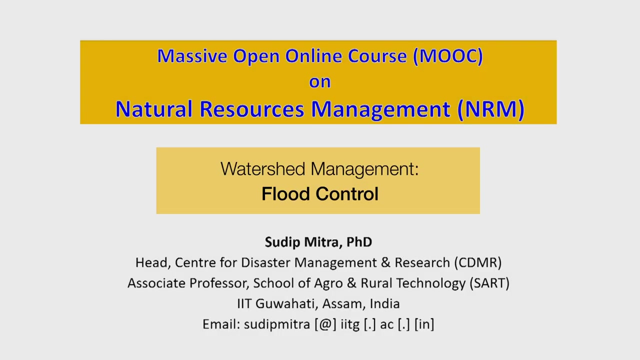 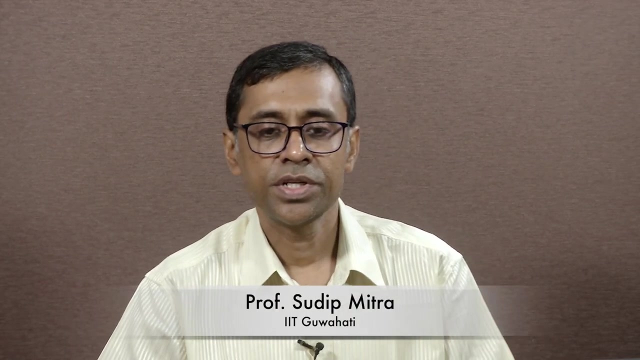 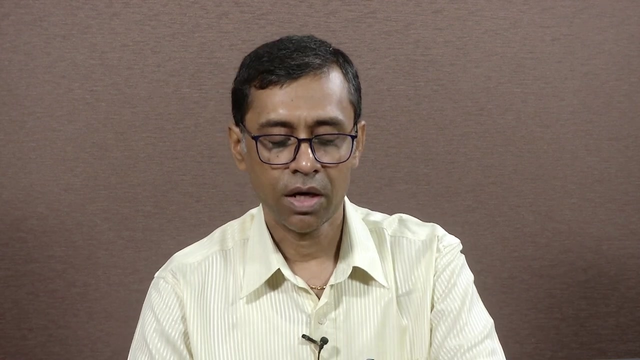 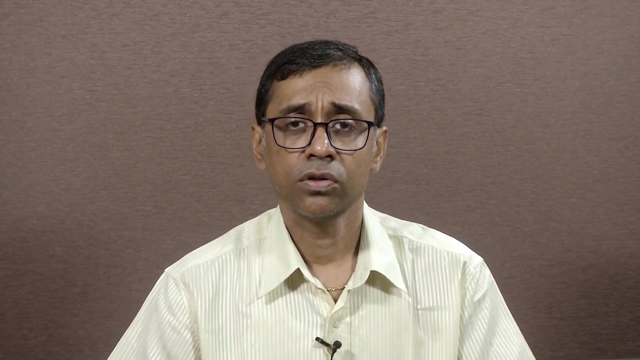 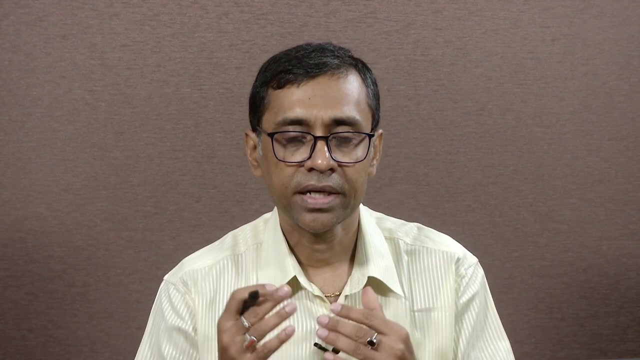 Next is flood control, And we discussed quite a lot about that: how actually we can restrict the soil erosion and, along with that, how we can actually conserve water and recharge also the groundwater. But in case of flood, also within a watershed area, it is important to actually also see how we can deal with floods. 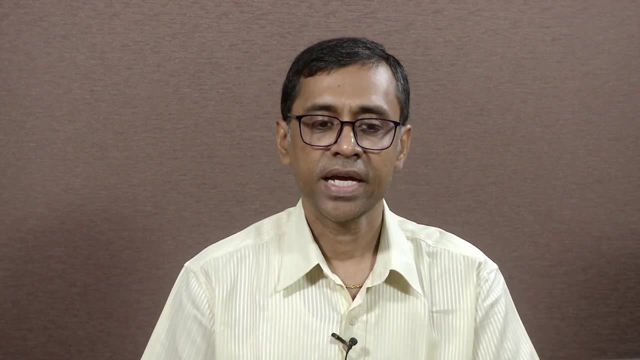 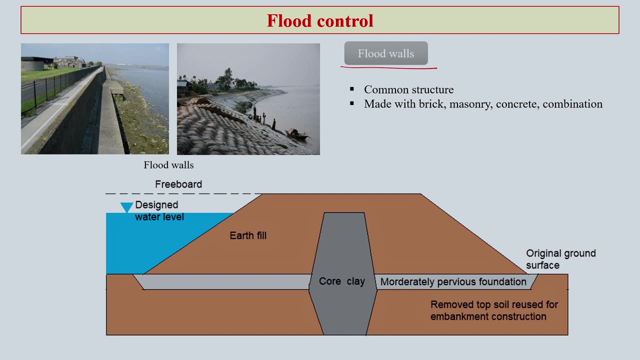 Now there are various ways that flood can be managed. One is flood walls, which is one of the most common way, common structure that we see in and around us, normally made with brick, masonry, concrete or combination of all those things. 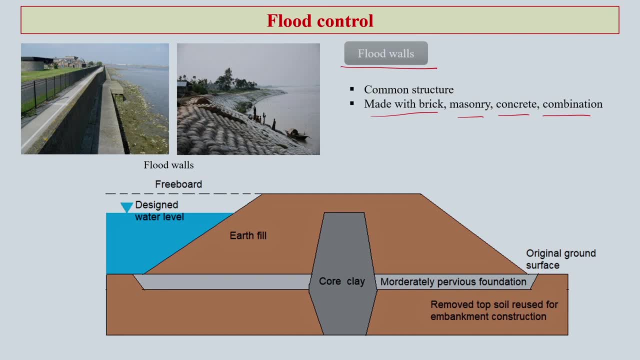 Even, sometime, sand bags are also being used. How it is actually basically done is that you have kind of a suppose that water level up to this range And then you try to have flood, First, earth filling, and then you go for, you know, try to make the height of this earth filling in such a way that it can also, you know, take care of the original ground surface. 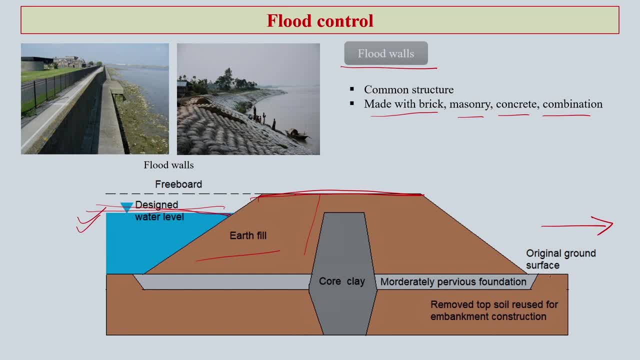 The original ground surface is basically the surface area which has the topsoil, where actually majority of the agricultural purposes or agricultural practices will be carried out. The removed topsoil, what is being done here? that it is reused for the embankment construction. 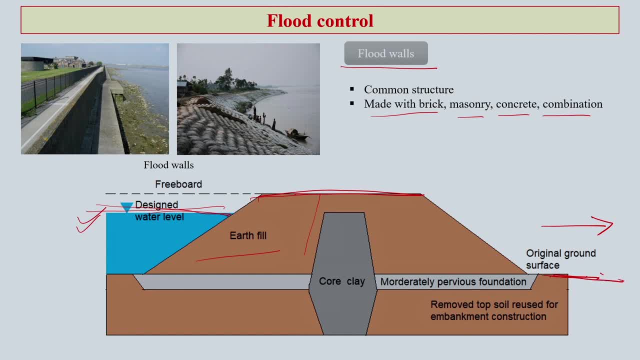 So you don't allow the topsoil to go away, You bring in back and do the filling with that soil which otherwise could have lost from the system. So this kind of earth filling also quite common, And this is done to avoid floods. 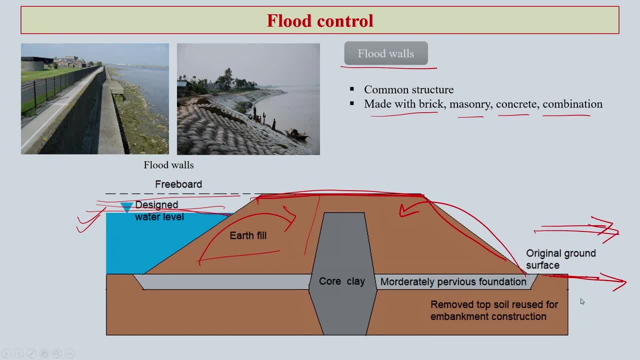 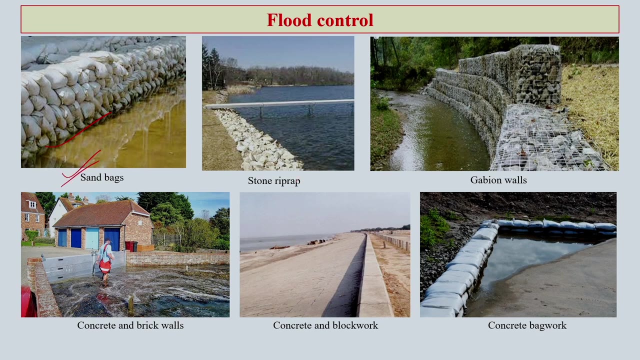 And this is done to avoid flood or impact of flood severely on the other side where habitation and also agricultural practices are going on. But of course we know that beyond a certain point this kind of structure also may not work. Sand bag- this you have seen many places- stones, riprap also are being used along the side of the river. 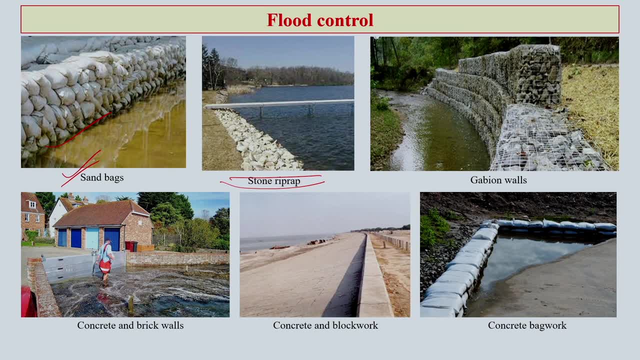 Then gabion walls also are here used. If you anticipate that your water level is going to be reduced- Your water level could actually rise with the rainy season- Then concrete and brick walls are often used, And these are seen largely in the developed countries. 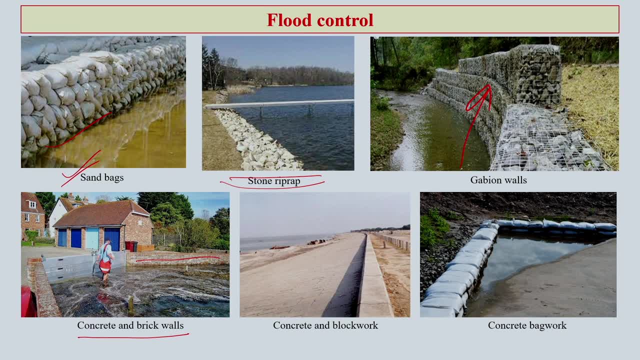 And sometime also you can see in some coastal regions of India in a different format. Concrete and block work. These are also visible in many parts of our countries along the sea coast. Concrete and block work: These are also visible in many parts of our countries along the sea coast. 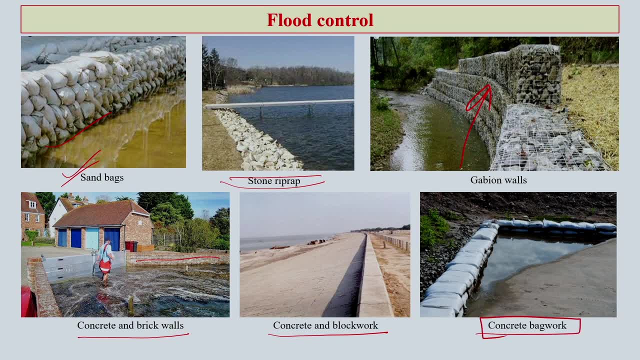 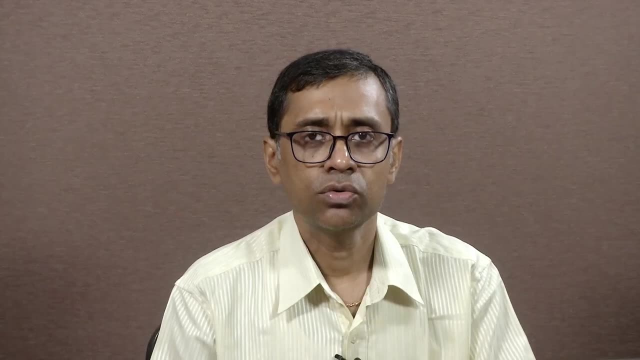 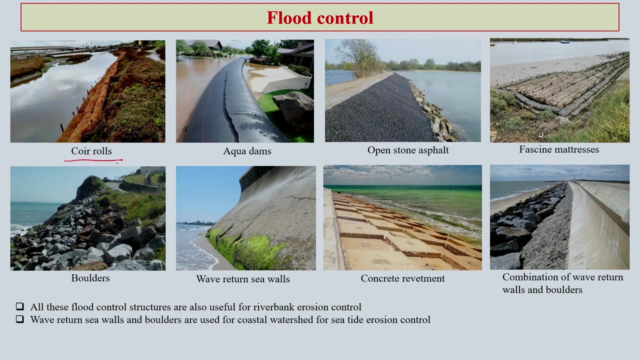 bag work is another option that people these days use quite a lot. so we have this kind of options available with us to reduce the impact of a flood on the ecosystem one step ahead. if we want to go with the technology options, we have choir rolls also, which can be used as you see here you 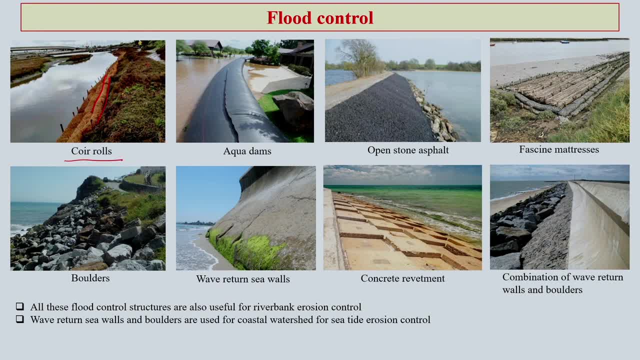 know the choirs that you get that can be made roll and then you can, across the slope, pack it so that if in case of rising of water it can actually get soaked there in this choir and then it actually also allows to the soil to get the appropriate amount of moisture. so this helps. 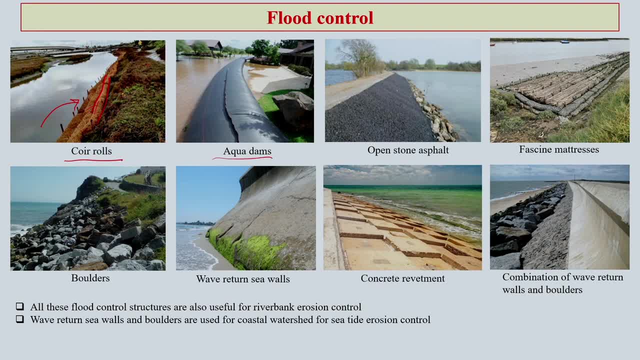 in both way. aqua dams is not, you know that, much common in our countries. open straw like this is not so common in our countries. open straw like this is not so common in our countries. asphalt also we may not see very frequently in our country. there are measures, like you know, boulders. 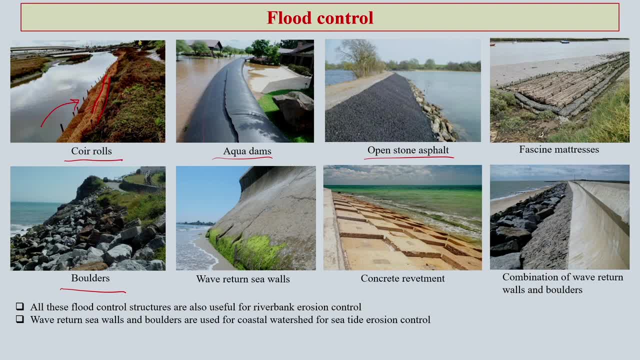 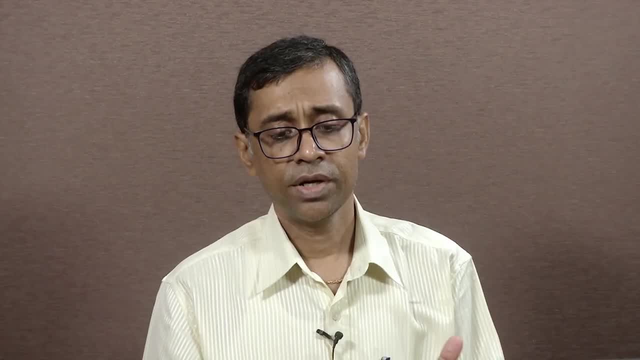 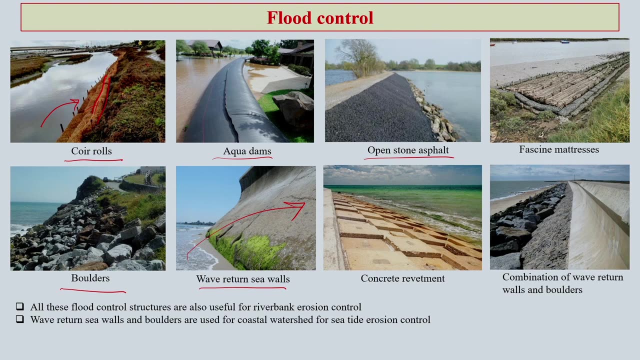 this is common in many places of our country as well: wave return sea walls. this you will see in marine drive area. so whenever there is, you know, tide comes, so the water actually hit these walls. so this somehow protect the civilians and also the inland agricultural purposes or any other you know human related activities, concrete revetment: this also reduces the flow. 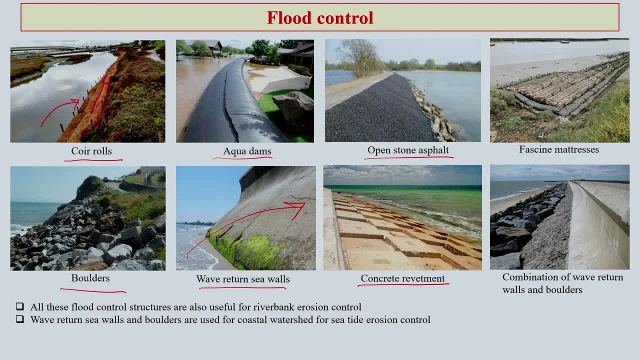 of water as well as the soil loss from the particular affected area. so the flood water if it comes, you know, suddenly, then it, the flow of water, can be reduced quite significantly by concrete revetment combination of wave return walls and boulders. this is not, again, very common. 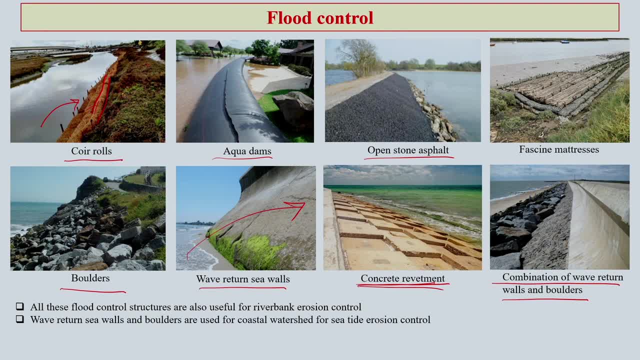 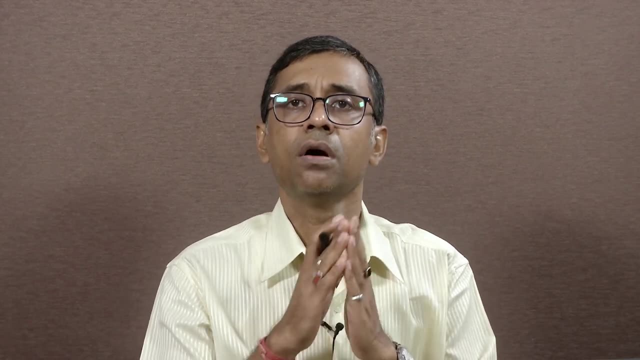 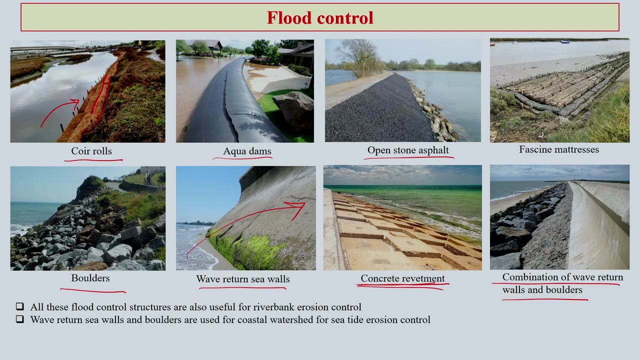 in our country, but is an another. you know, potential techniques can be used across the coastal line. all these flood control measures are also useful for riverbank erosion control. so this is why, actually, i am sharing all the options that you know in across the world people use. so it is kind of a basket of options that i'm trying to share with you. 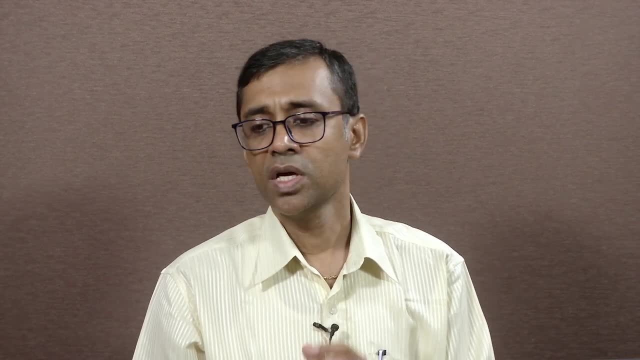 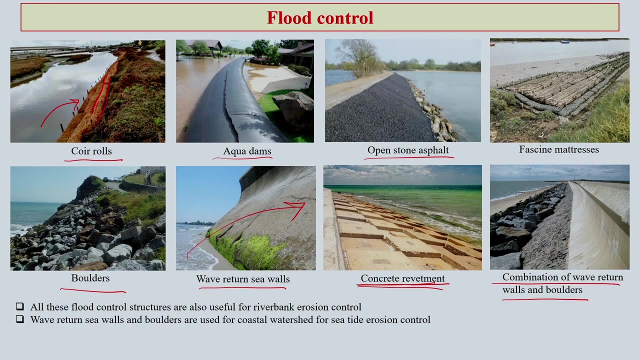 given, you know, situation and and opportunities. some of these options can also be utilized, as i said that, for riverbank erosion, but wave written sea walls and boulders, these two, you know, are used for coastal watershed mainly and to reduce the sea tide erosion control. okay, so we have actually a lot of technological options with us to also, you know, to 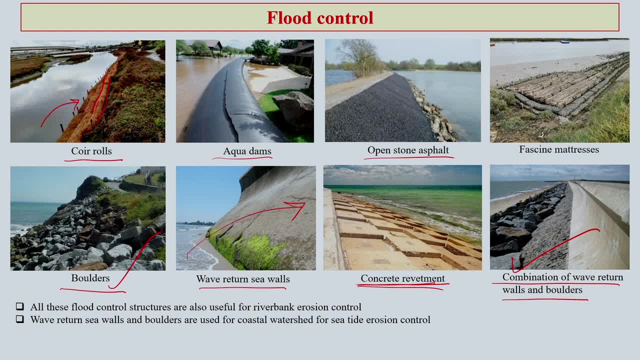 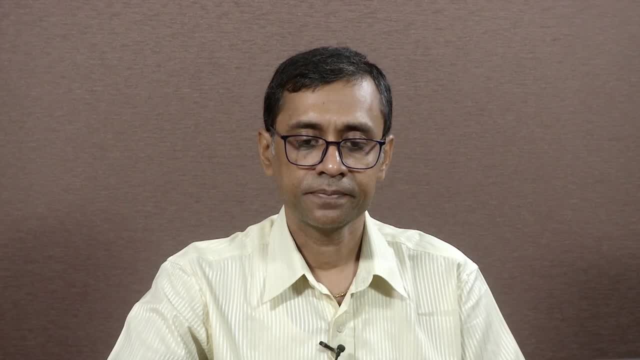 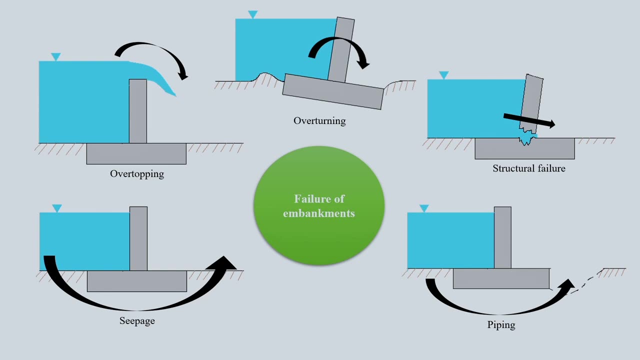 reduce the impact of flood. but we may not be able to totally stop it, but the effect can certainly be reduced if proper measures are taken. now why? we listen quite often that embankments have failed to do its job. if the embankment has done with all right technology, why then it fails? 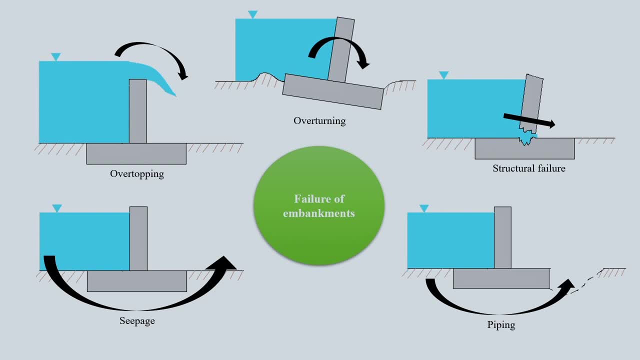 now there are various regions for that. some of those regions i would like to discuss here. one is that over topping, as you see that the embankment has been made but the water amount of water coming into the system is so high, the volume is so high. 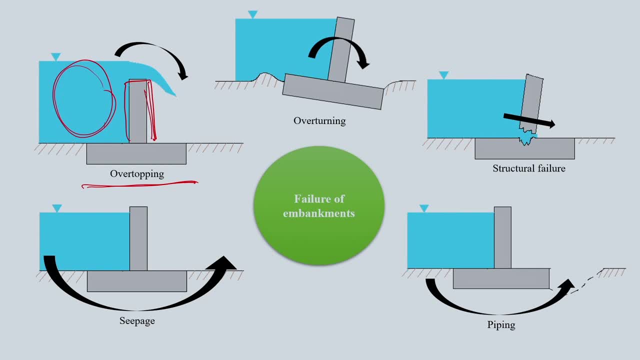 that even when you have built this embankment you actually anticipate, certain amount of assumptions are involved that how much water actually, even in maximum, you know rainy season could come up. but if your that assumption also is, you know, failed or means it crosses beyond even that limit, then 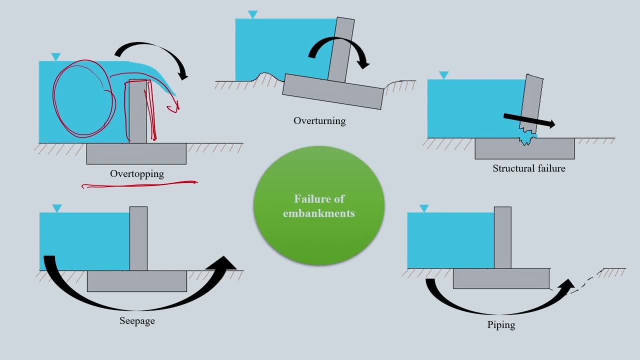 certainly the water will flow above your embankment- and this kind of situation are actually rare, but this can happen- and in that case your embankment in actually fails to do its job. second case is overturning. what happened is that some time, because of certain movement in the soil or, along with that, the again amount of water, 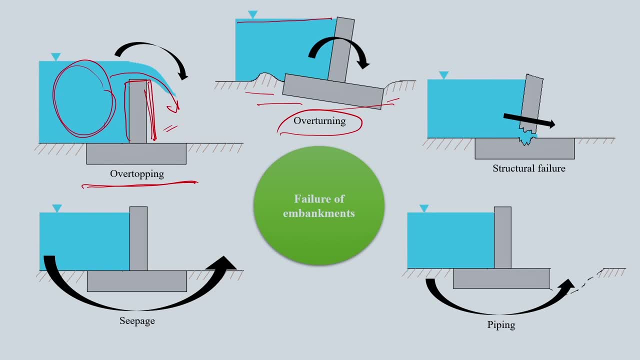 if sudden flow of water increases heavily, then there is a chance that your embankment structure can be overturned, and this kind of situation we often see in many cases in and around us. so that is another point that we should keep in mind while establishing this kind of embankment. 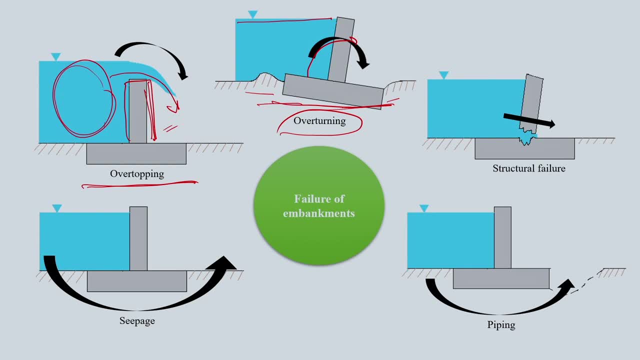 that overturning of environment can also take place. structural failure, that's purely, you know, technological engineering failure which can certainly be avoided, if not 100, but at least engineering wise, technically, this can be easily rectified. so as you see here that there is a crack in the 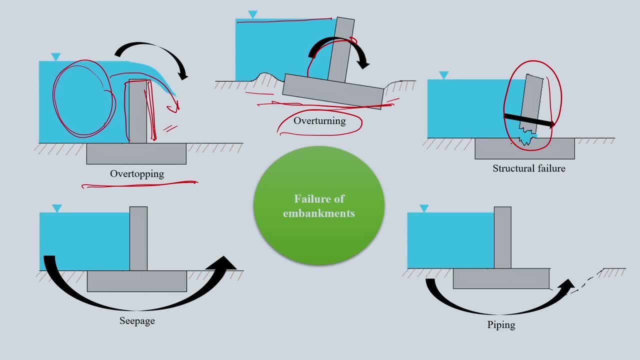 embankment structure, but, as i said, this can be avoided to a large extent. seepage: seepage is another issue that actually takes place very silently and often when we establish this kind of structure, we need to actually look into this aspect, that seepage can also takes place. so, due to seepage, 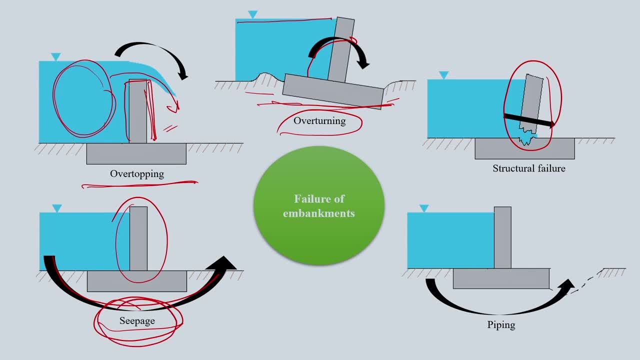 sometime our embankment structure also fails to do the job in appropriate manner, piping or peeping. so that is, you know, another problem, that sometime your embankment actually fails, and that sometimes happens for two reasons. one could be that it is not properly established. the ground verification was not done. 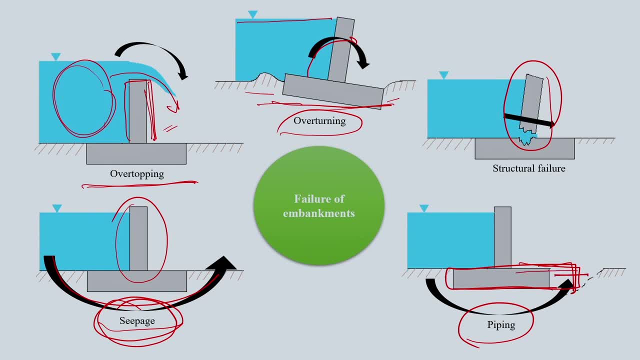 appropriately, because if you see that you have kept a huge amount of gap from your support system, sidewall support system, then there is a chance that water may actually, you know, cross your foundation of embankment and then can weaken this embankment structure. so these are few, actually. 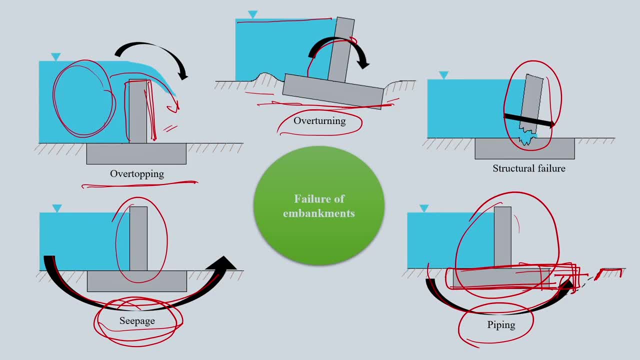 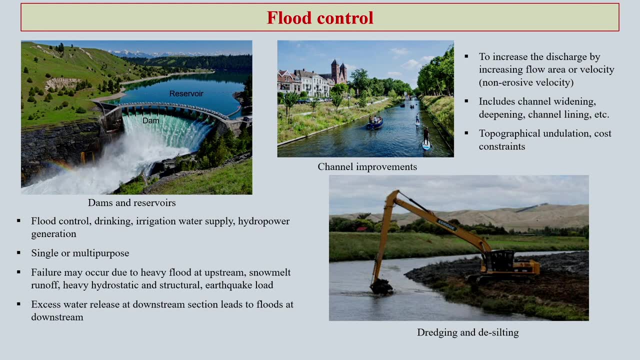 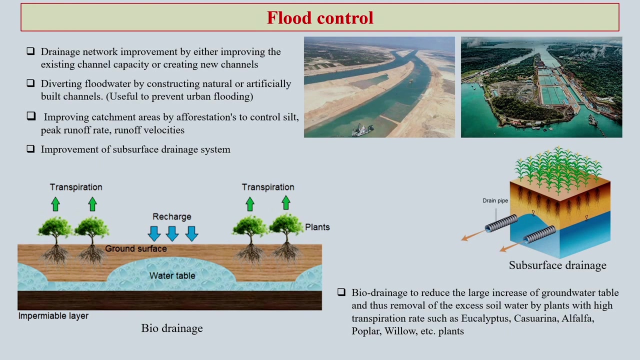 potential failures of embankment that sometime construct. so there are various other options also for fart cartel. these are reservoirs, dam channel improvements, drainage, dredging and desilting. all of those things are very common and i'm sure that all of you are quite well aware of. then comes. you know, these days bio mitigation is coming heavily and that 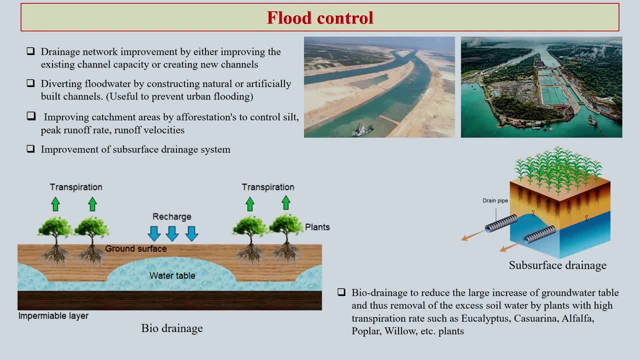 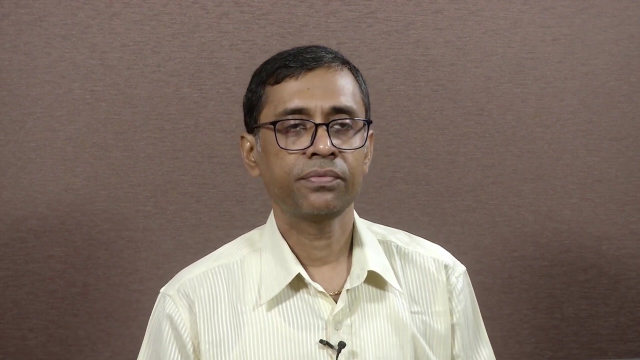 how actually you can utilize different kind of plant species and also how you can actually create a bio drainage system so that the drainage network can work in an appropriate manner. you can do it either improving the existing channel capacity or creating new channels. this can also be done by diverting the flood water by constructing natural or artificially built channels. 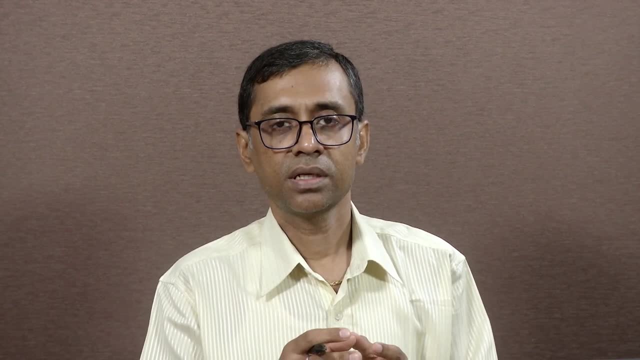 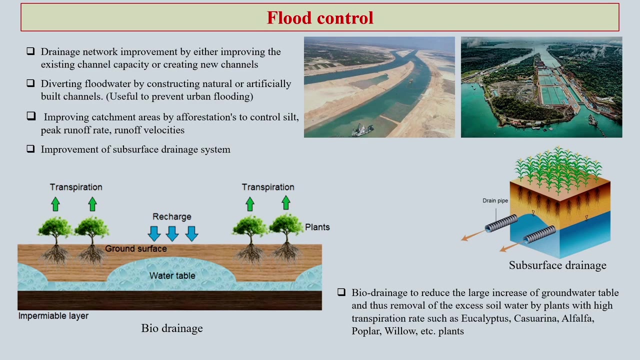 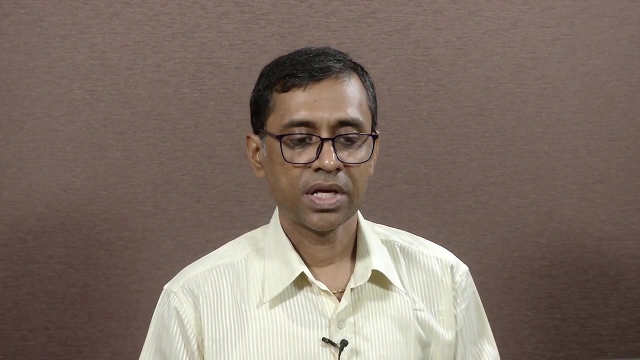 we can also do it, improving the catchment areas through afforestations to control the seal, the peak runoff and also the velocities of the water. improvement of subsurface drainage system is also critical. uh, you know, for flood control measures, as you see in. you know in this picture that you basically try to adjust. 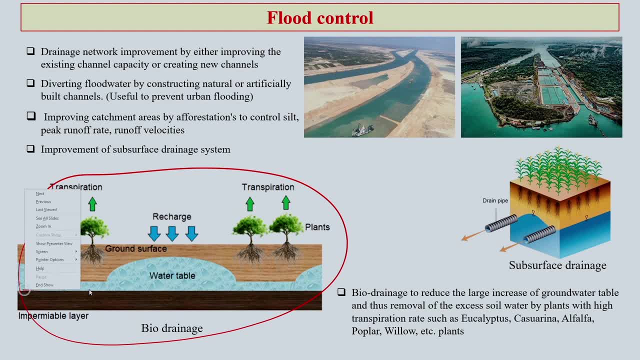 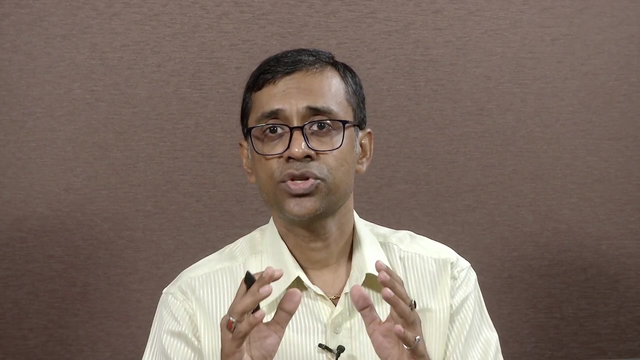 through different kind of plantations. the drainage system actually can be improved with the help of suitable plant species grown in and around the water table, that, through ground surface, the recharge of groundwater in a very regulated manner can take place. we use proper plantation, a proper plant species in an area. some of the species, as you know, like: 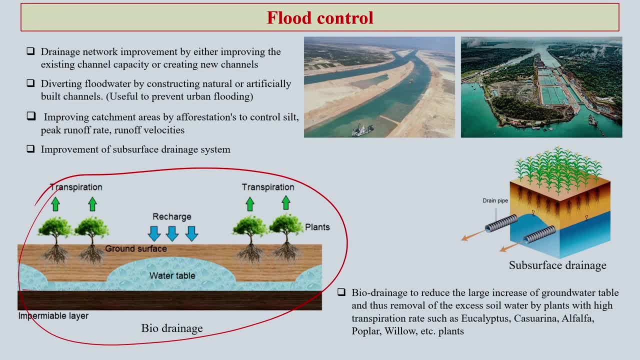 vetiver works very good, not only for soil strengthening soil, you know- structure improvement, but also it, you know, has its own inputs into the soil for improving its quality. so it not only reduces flow of water, soil erosion, but also it can get rid of many other kind of 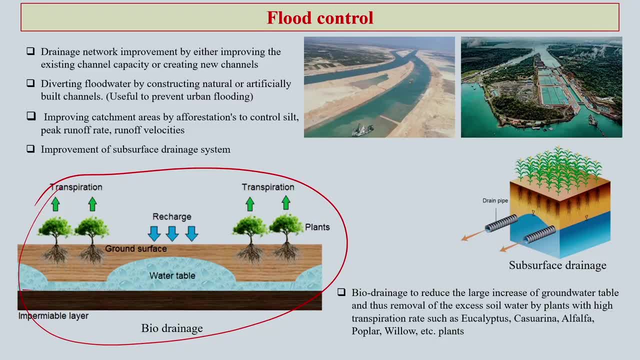 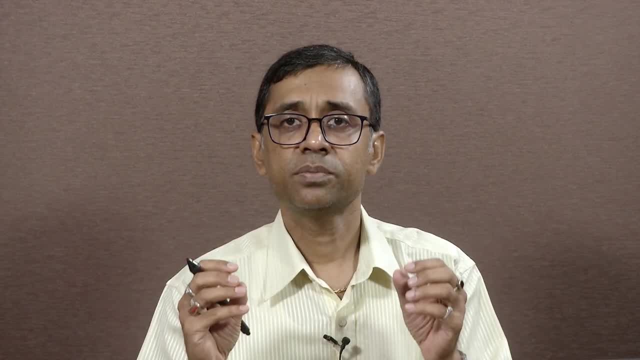 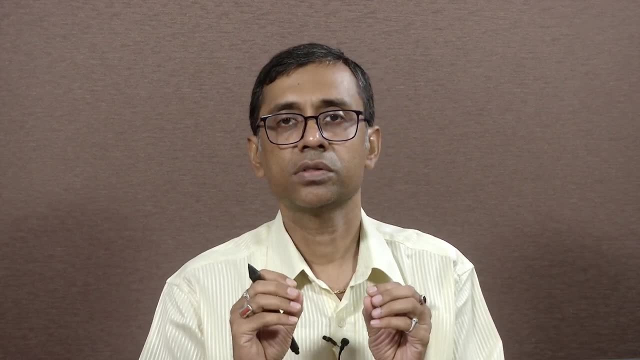 also provide some inputs into the soil and also enhances the microbial activity dynamics in the soil. So in a sense that a plant species, if it is properly chosen, it not only reduces the impact of flood, it not only reduces the soil loss but at the same time can also- you know- provide some other. 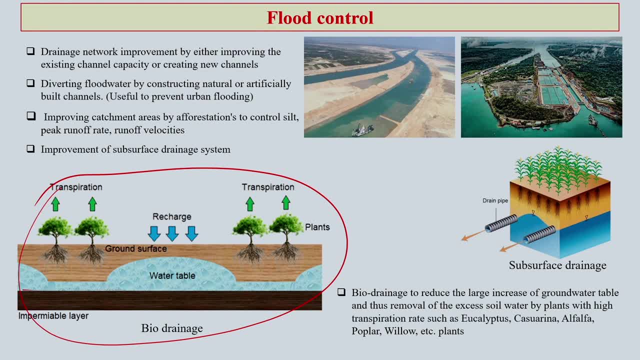 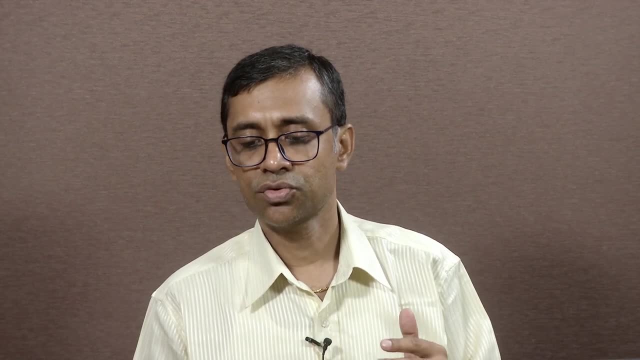 ancillary benefits. Biodrainage also reduce, you know, the large increase of groundwater table and thus it can help in removing the excess soil water by plants with high transpiration rate. So, such as you know, sometime you will see eucalyptus casuarina, alfalfa, poplar willow. 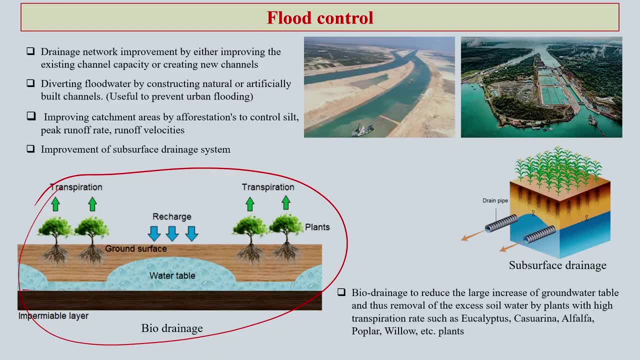 these kind of plants are often used, But this kind of technology also has to be done with proper investigation on the ground level, As I said that choosing of appropriate plants for particular area is critical, Because every plant cannot be or should not be used in any area without the ground verification. 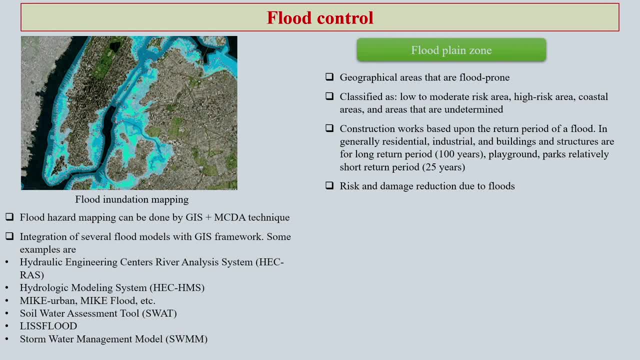 Now continuing with flood control. flood plain zone, I know, is very important, and flood inundation mapping through GIS and remote sensing these days help us to actually identify the exact area, that which are the area is actually is affected, and then various kind of you know engineering technologies can be used for development or further improvement of flood affected area.